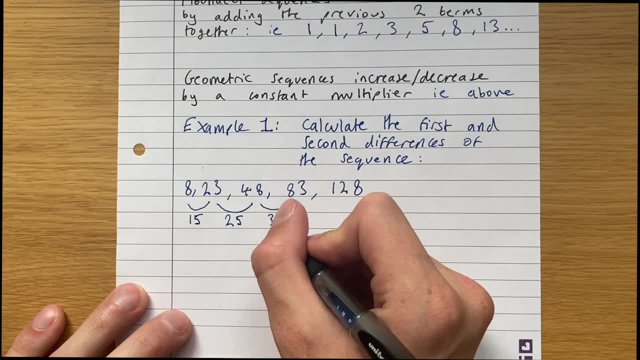 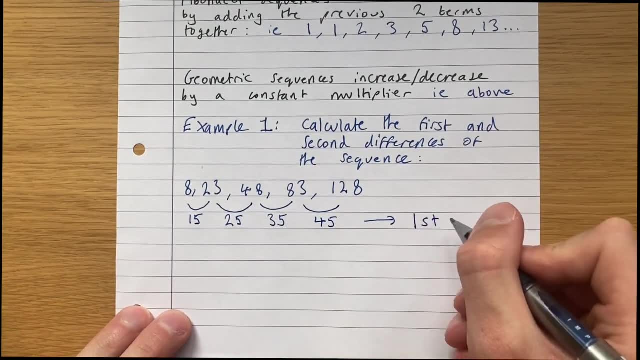 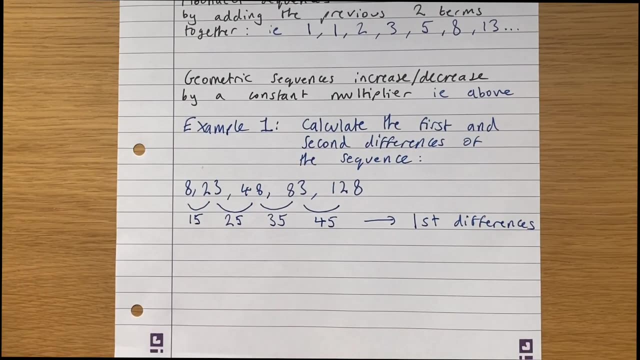 48 and 83 is 35.. 83 and 128 is 45. These are what's known as the first differences, And the second differences are just the differences between the first differences. So the difference between 15 and 25 is 10, 10, 10.. And that those are the second differences And these 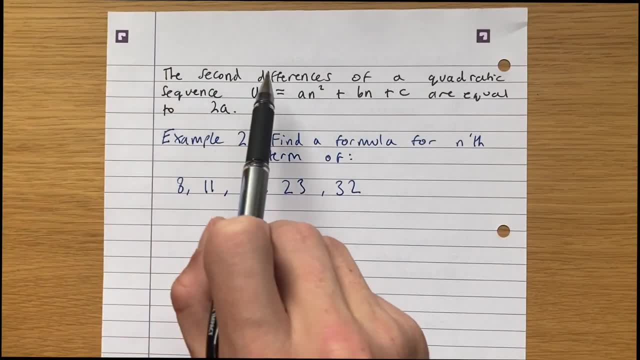 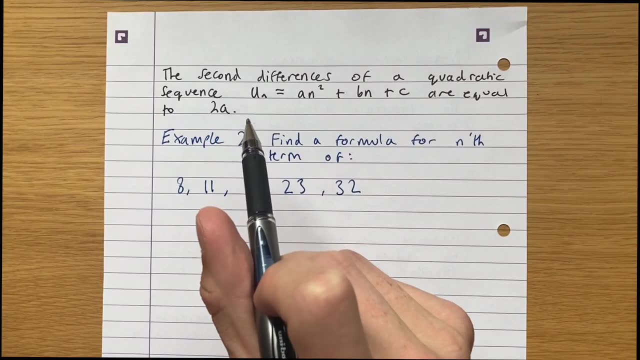 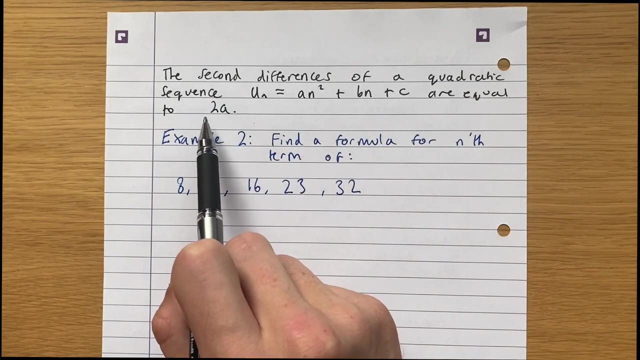 are going to be very useful later on. So the second differences of a quadratic sequence, meaning the highest power is squared. that's what quadratic means. The second differences of a quadratic sequence: un equals an squared, plus bn plus c are equal to 2a, And this 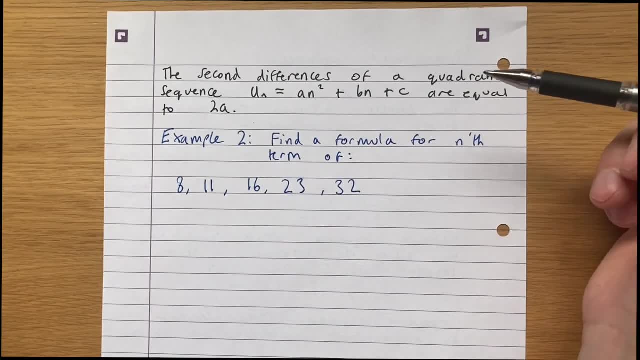 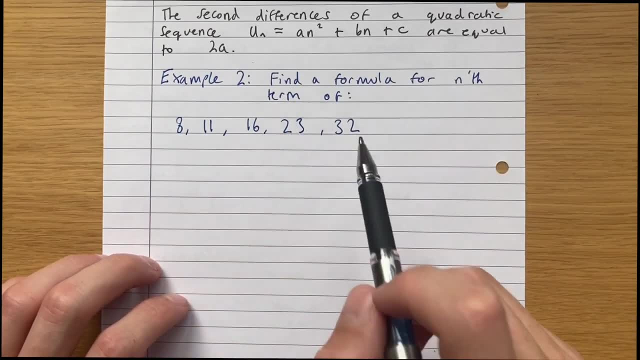 is really useful when we're trying to find formulas for the nth term. So we'll do an example to illustrate this now. So we're finding a formula for the nth term of this sequence: 8,, 11,, 16,, 23,, 32.. 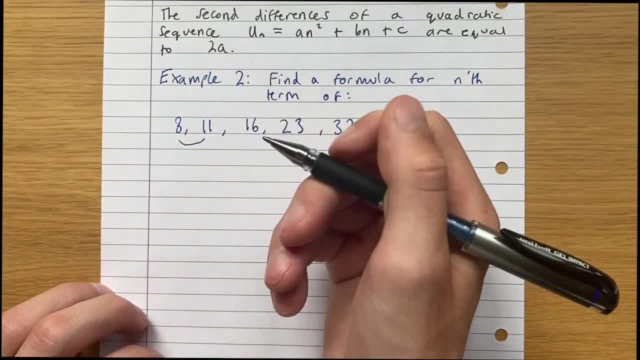 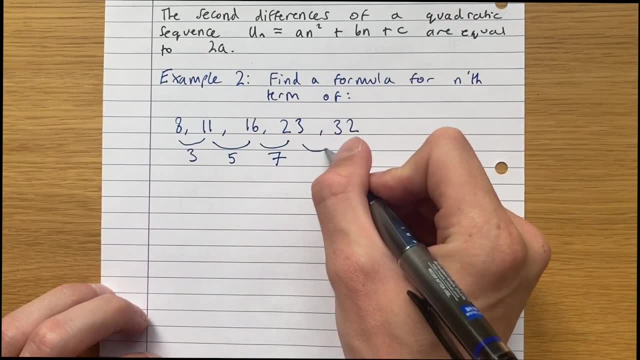 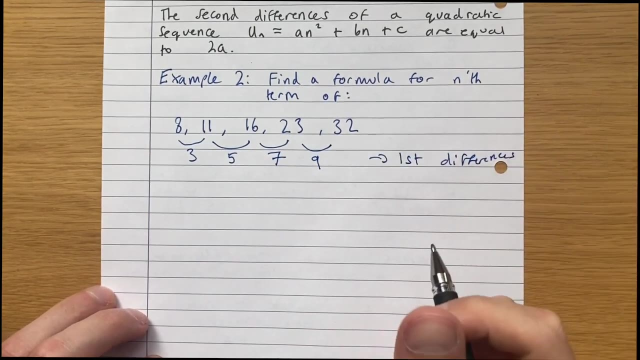 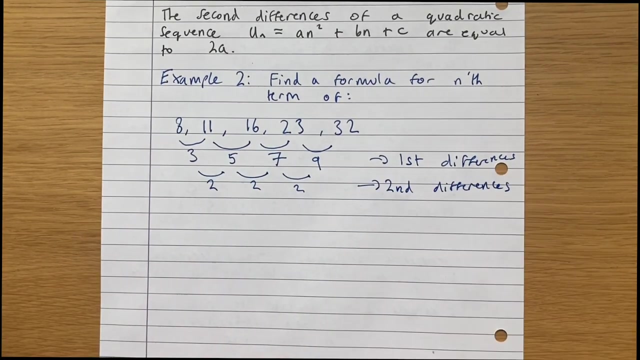 For questions like these, you always want to find the first and second differences with non-linear sequences. So the difference here is 3, then 5, then 7,, then 9.. So those are the first differences, And the second differences is just 2.. All of these are different by 2.. 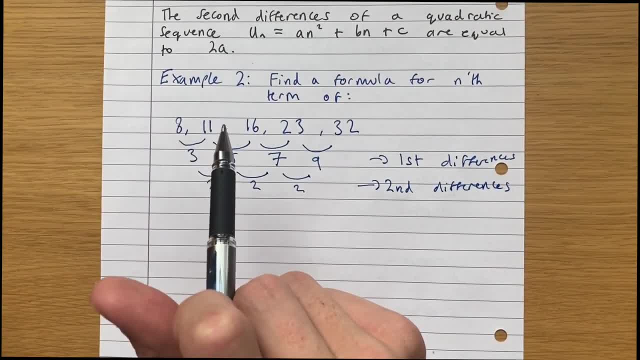 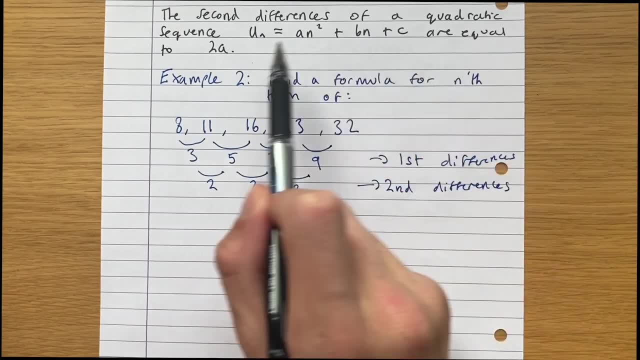 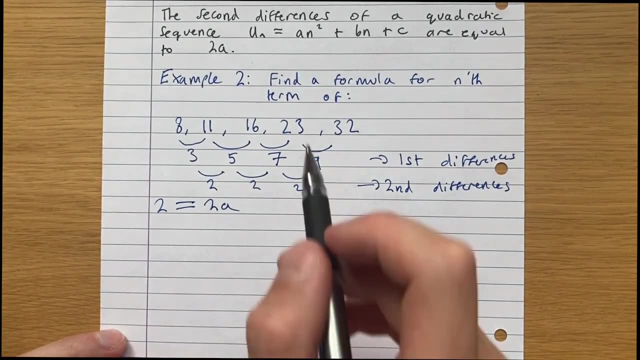 So this is where what I've written above comes into play. The second differences of a quadratic sequence: un equals an squared. plus bn plus c are equal to 2a. In other words, 2 is equal to 2a in our sequence. 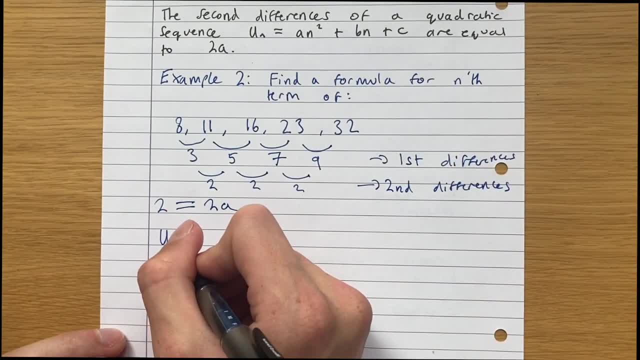 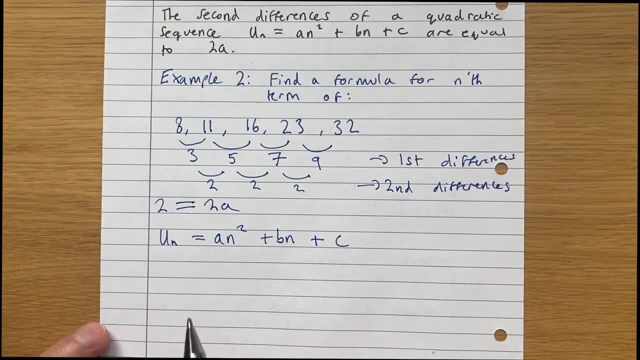 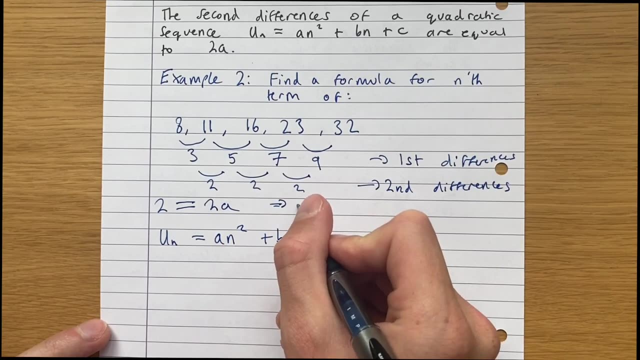 So we're trying to find the formula for the nth term. So we know it's going to be of the form: un equals an squared plus bn plus c, And we're told here that 2 is equal to 2a, So this just means that a equals 1.. So we know that our sequence is of the form un equals. 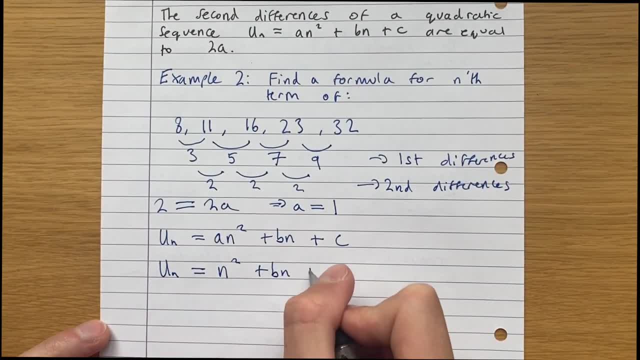 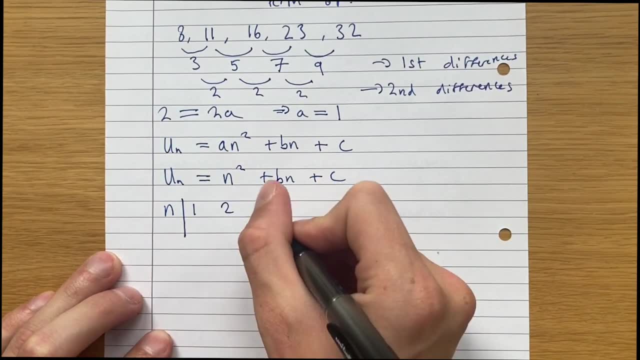 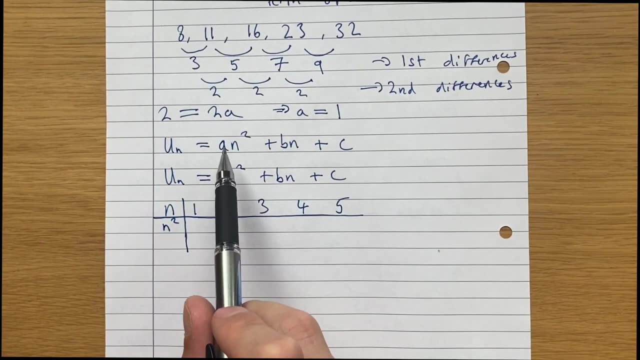 1n squared plus bn plus c. So if we write out, if we do a table again: so n 1,, 2,, 3,, 4,, 5. And so n squared, we know that a is 1.. If un is n squared, we just get 1.. So we're. 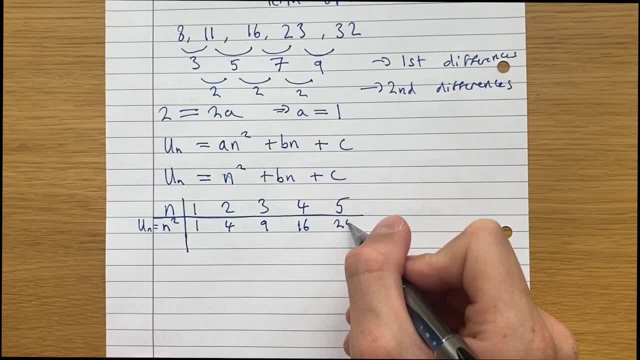 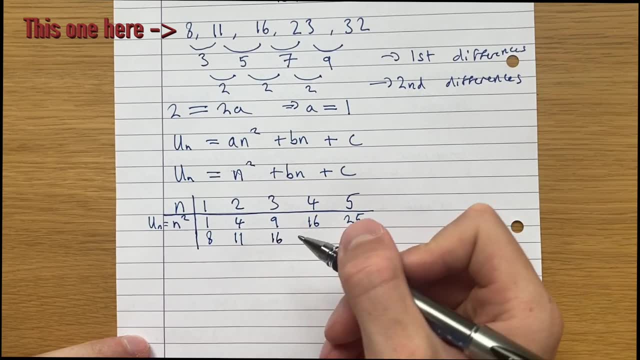 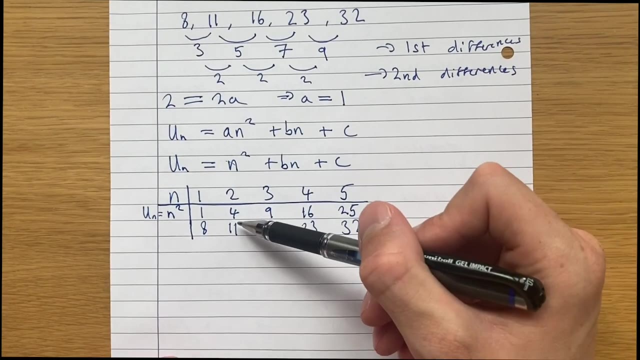 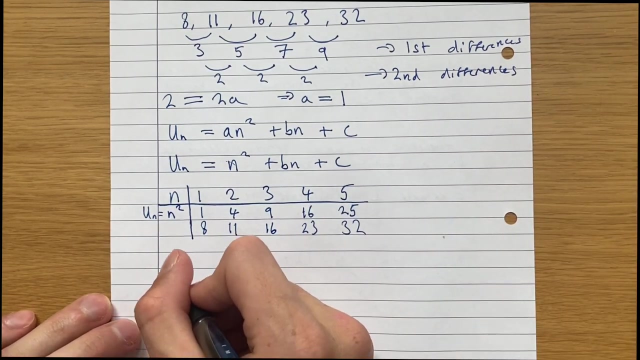 going to get 1,, 4,, 9,, 16,, 25.. And our actual sequence is 8,, 11,, 16,, 23,, 32.. Just by inspection, we can see that the difference between the terms here is just 7.. Right, So what we get? 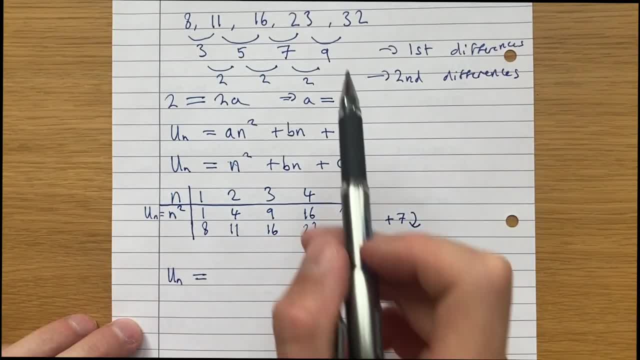 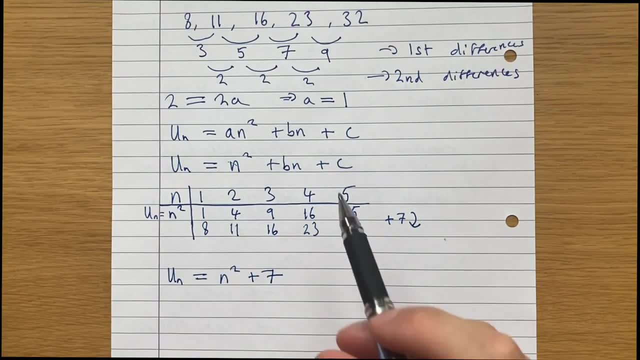 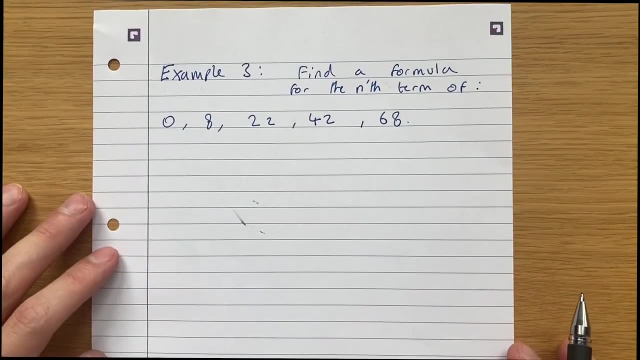 is just plus 7.. Because you're just adding 7 to get to our sequence from n squared. So un is equal to n squared plus 7.. So in this example it just so happened that b was equal to 0, which made life somewhat easier. So now let's go through an example where b is: 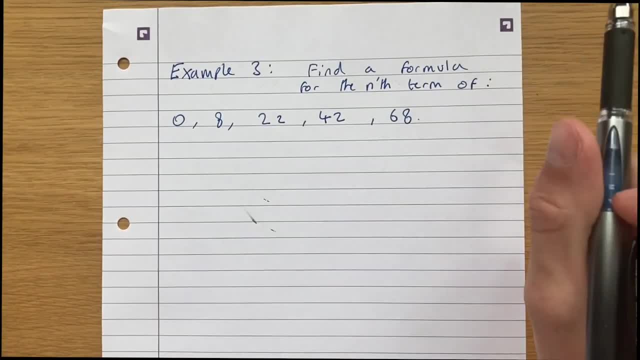 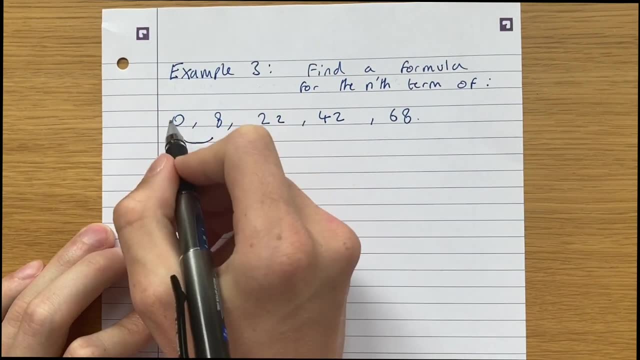 non-zero and how we go about solving that. So similar question: We're finding a formula for the nth term of this nonlinear sequence. So you do the same thing as always: You find the first difference, You find the first difference, You find the first difference, You find the. 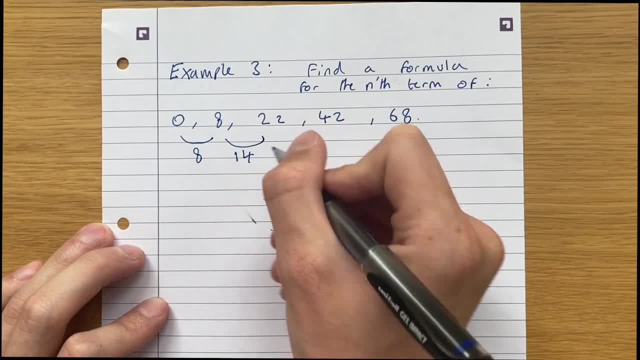 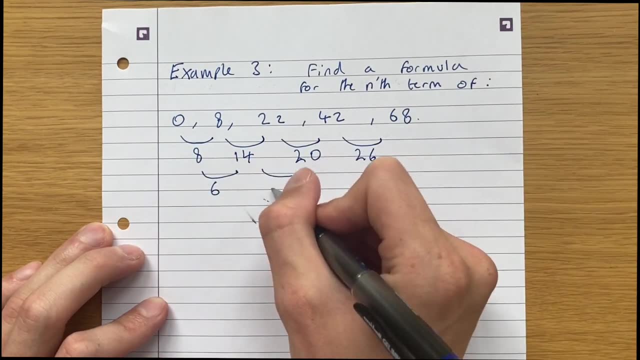 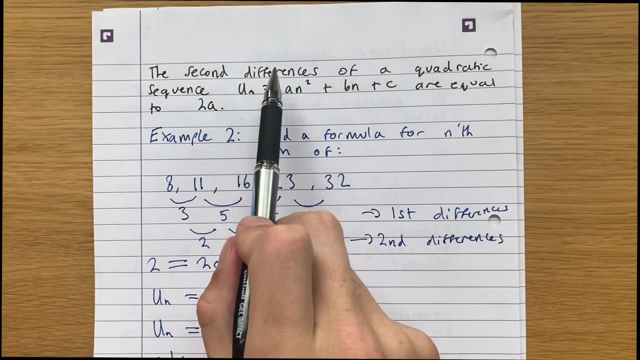 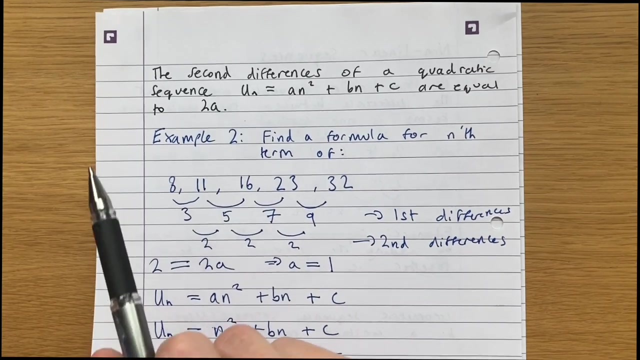 second difference. You find the second difference, So 8,, 14,, 20,, 26.. The second difference is being 6,, 6,, 6.. And if we just remember our important fact, the second differences of a quadratic sequence: un equals a, n squared plus b, n plus c are equal to 2 times a In. 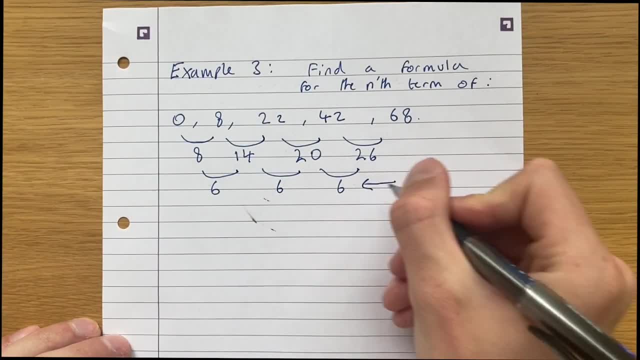 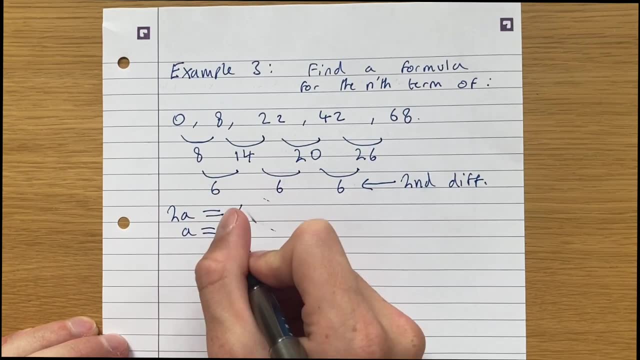 other words, our second differences are equal to 2n squared plus b, n plus c. In other words, our second differences are equal to 2a. So 2a is equal to 6.. So a must be 3.. Our expression: 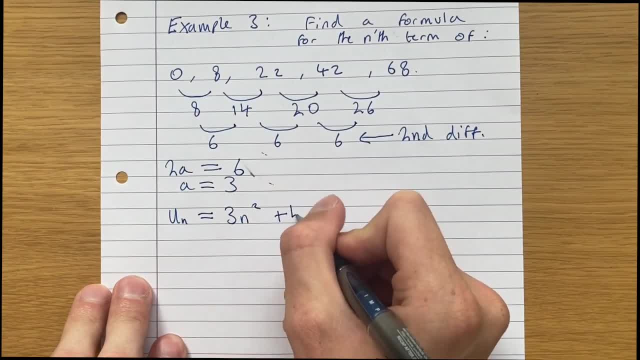 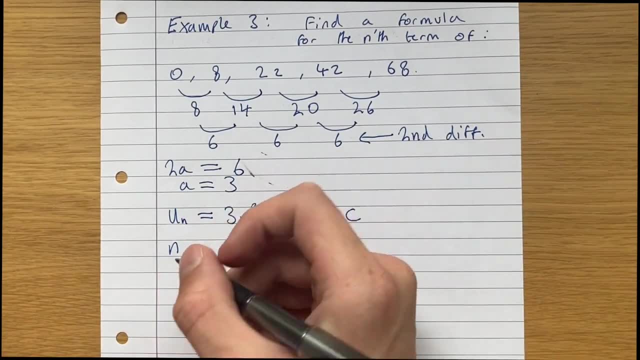 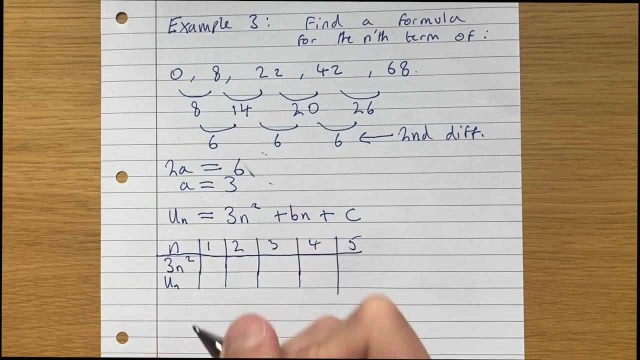 for un is of the form 3n squared plus b, n plus c. So if we do the same thing we did before, we write out n, we write out 3n squared, and our sequence, which we're trying to find the expression for. 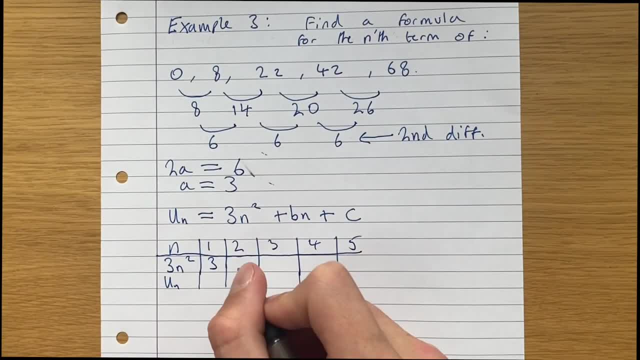 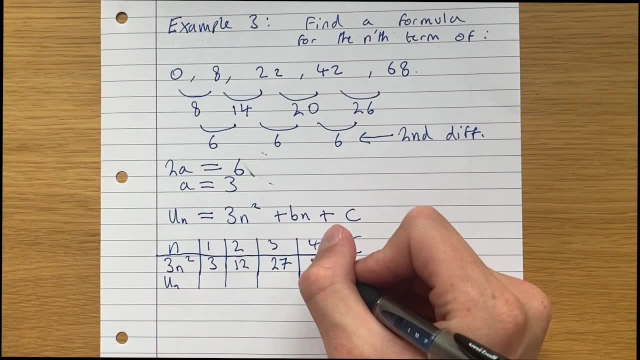 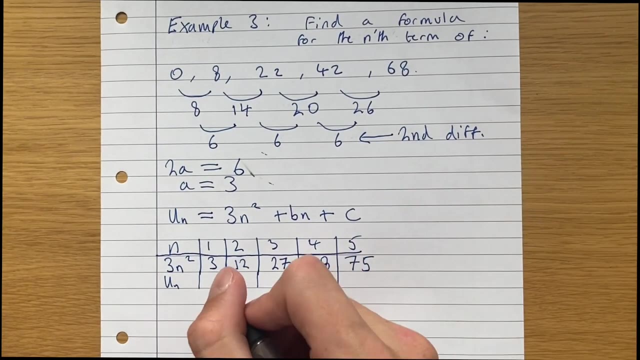 So 3n squared would just be: 3 times 1 squared is 3.. 3 times 2 squared is 12.. 3 times 3 squared is 27.. 3 times 4 squared is 48.. And 3 times 5 squared is 75.. And our sequence is 0, 8,.